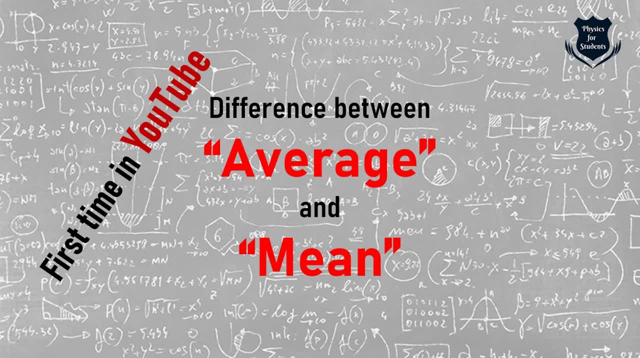 But it just came to my mind that what could be the difference between calculating the average and mean, like what those two terms actually mean? If they give the same results, then what is the use of using those two terms in mathematics? So welcome everyone to this new video, and I am trying to show you the fundamental and the conceptual difference between calculating an average and a mean. 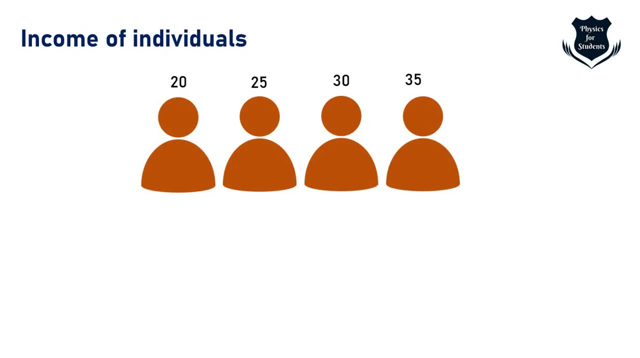 In general, if we take the income of individuals, say, for example, 20,000.. 25,, 30 and 35. I am not taking whether they are INR or Yen or Dollar or whatever, We just take the income of those individuals. 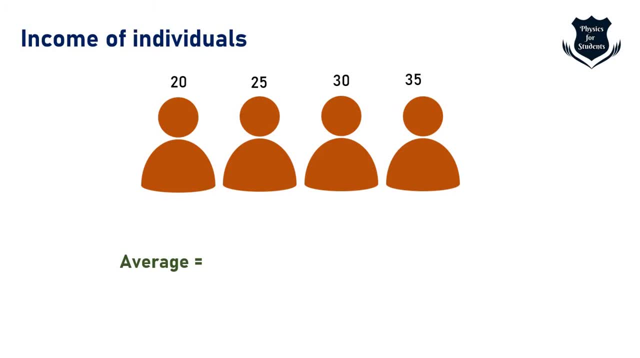 Then what we learnt in our school days? that if we calculate the average, we sum this up and then what we do is divide by the number of occurrences, which gives to this result 27.5.. This arrow right in the middle of your screen which points downward and is marked in red, 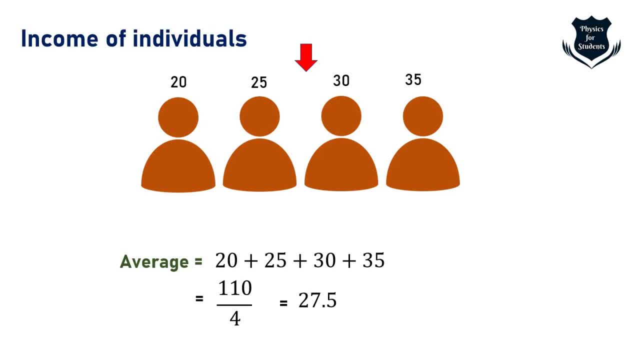 This is actually showing the average. This is showing the position. So this is what we know as how do we calculate the average of individuals, income of individuals. I have shown on the right hand side of your screen you can see, using the sigma notation, the formula of the same average calculation. 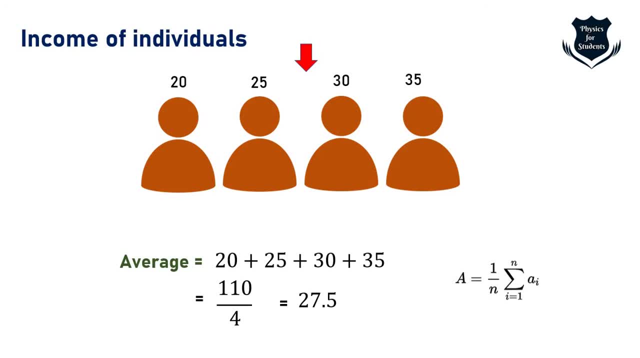 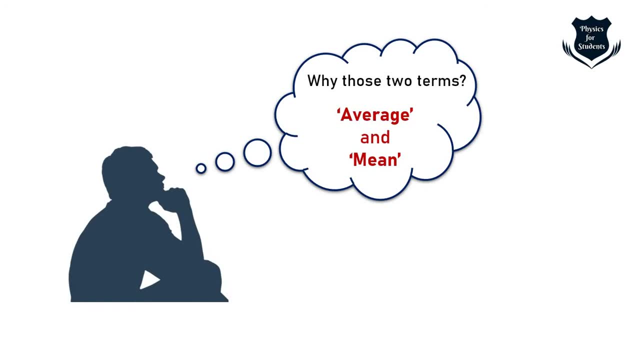 I have used this term so that it can go up to the calculating the value, up to the ith term. So why these two terms average and mean? Well, you need to understand one thing: That average actually is a very important term. The term average actually is a very misleading term. 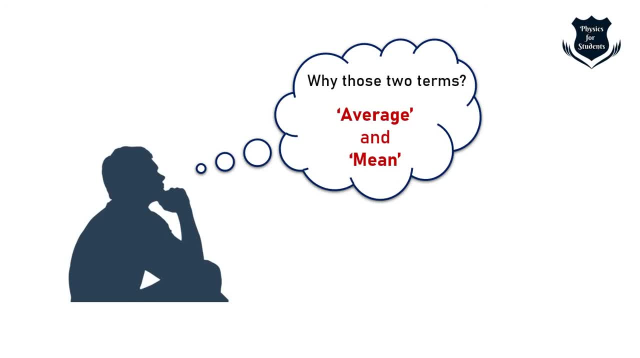 As you know that in the world of mathematics terms often are misleading. Why? Because what is understood in general in layman's word is not the same thing, or precisely, it is not the same value or the meaning what it is in the mathematical world. 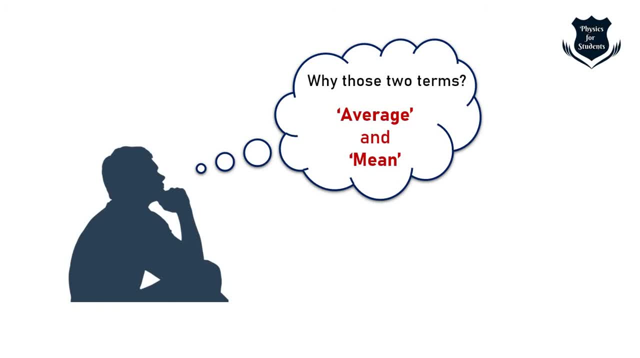 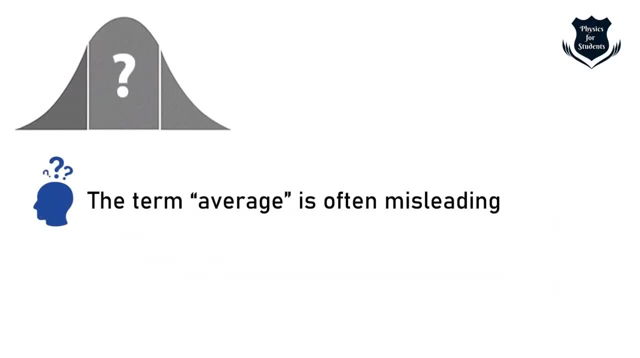 So we will soon see in this video that average and mean actually has two different meanings and why we use those two terms. Now, in general, the first point that we have to remember is that the term average and mean is not the same thing. The second point that we have to remember is that the term average is often misleading because it is a layman's terms and it doesn't signify anything precisely. 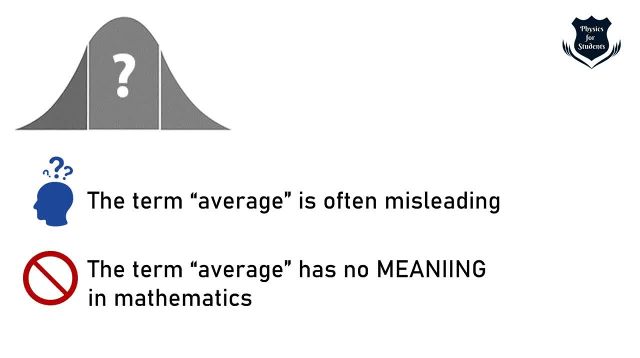 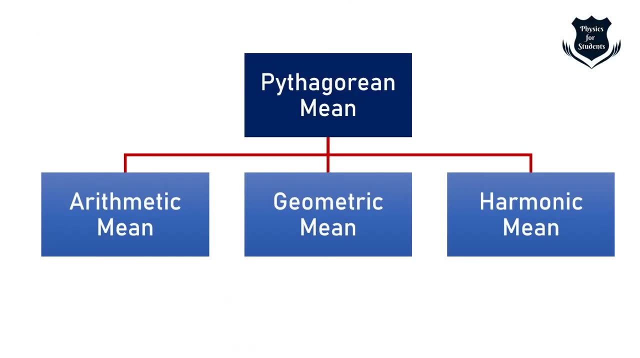 The term average has no meaning in mathematics, which will actually become more clear as we proceed with the video. So we have to be very careful when using these terms. average Now, as you can see in the screen of this hierarchy, Pythagorean mean has three meanings. 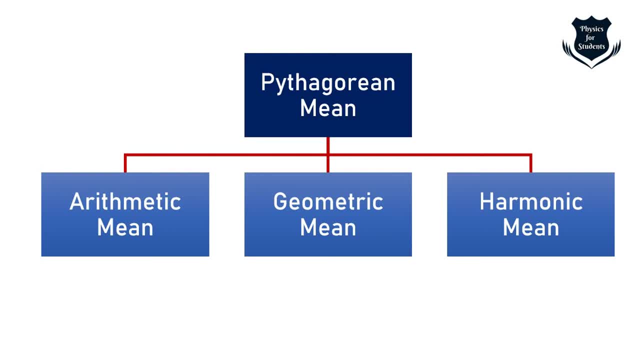 Pythagorean mean has three different branches: Arithmetic mean, geometric mean, harmonic mean. I am not going to go into details about geometric and harmonic mean and the formulas and calculations which you already know, But when we get forward and proceed and get a series like this which is 1 plus 2 plus 3 plus 4 plus 5.. 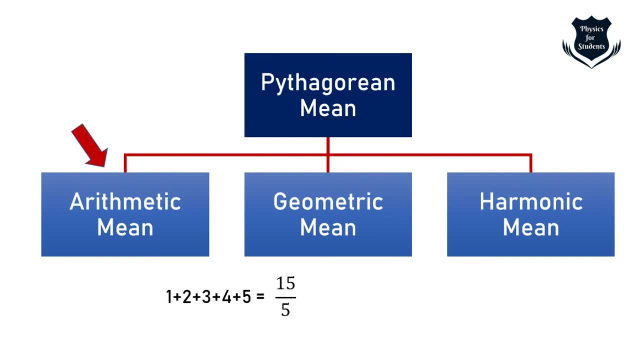 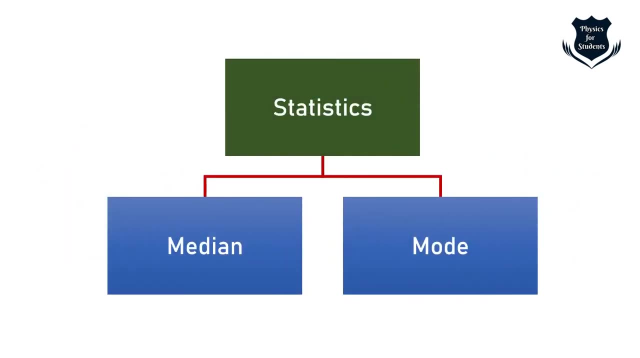 In general, when we take the average, what we mean is this arithmetic mean. So, as I told you that average and mean are misleading, So when we are meaning average, We are actually trying to mean what is an arithmetic mean? Statistics also have two branches, like two ways. 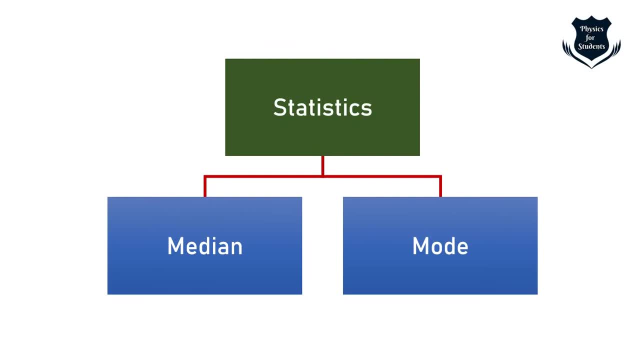 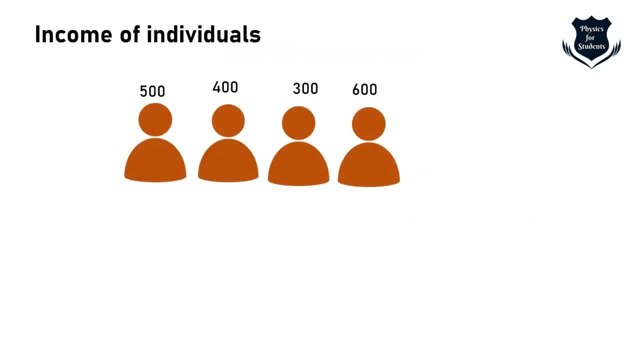 One is median mode. We will soon see what actually these two mean. So let us take an example: The same income of individuals. The numbers are 500, 400, 300, 600. And what is happening is that a new person, marked in blue, is plugging in whose income is 20,000. 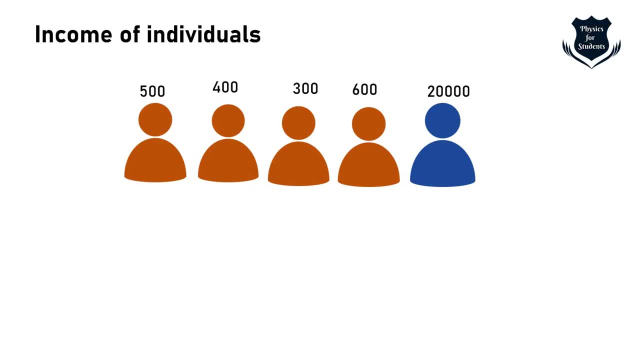 Now let us go back to our school days And get back to the textbook and calculate the average. So what we do is that we add up the same values: 500 plus 400 plus 300 plus 600 plus 20,000.. 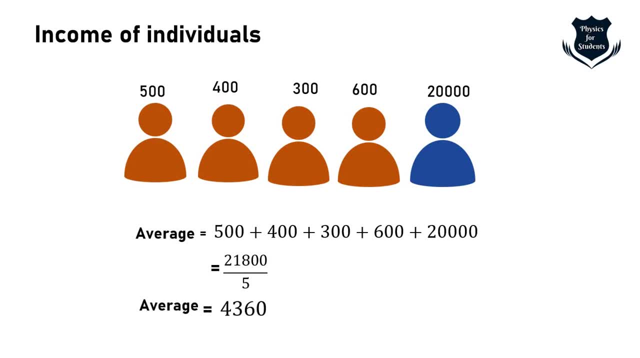 And divide by the number of occurrences, That is 5.. What we get is this: 4360.. Now, this is something which is wrong. Why? Because we all know When we get this value, 4360.. Where do we put in? 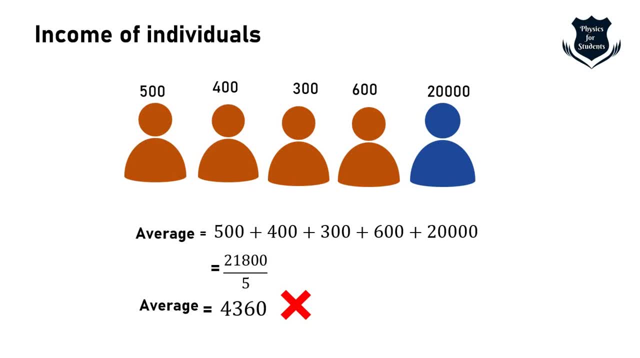 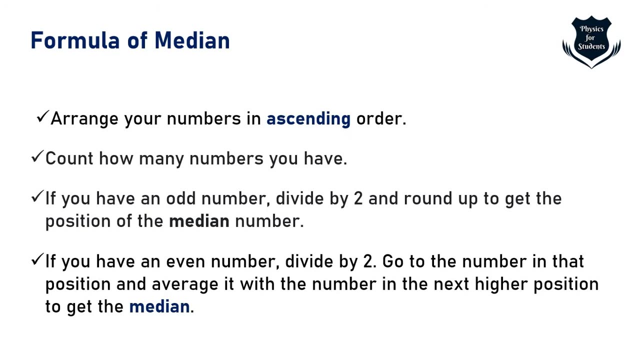 Something between 600 and 20,000.. Where is that point? No, It is not right. So this is not the way in which the answer for this average calculation should be done. So where do we go? We go here, We follow what we is that calculation of a median. 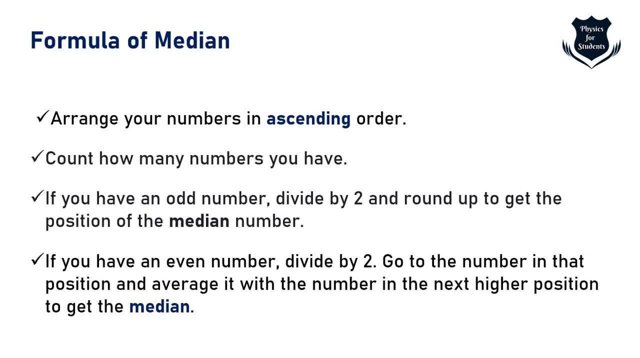 So we all know that we arrange these numbers in ascending order. We count the numbers we have. If it is an odd number, We divide it by 2. And round it up to get the position. And if it is an even number, 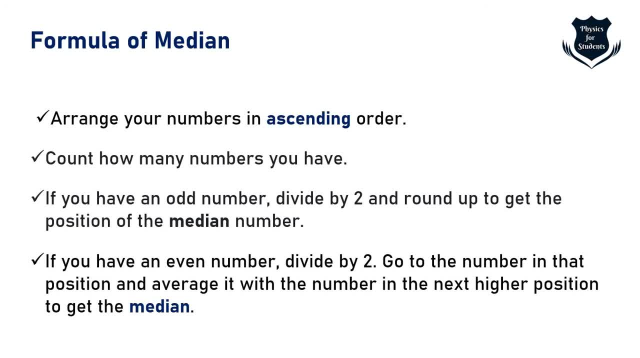 We divide it by 2. And go to the number in the position And average it with the number in the next higher position To get the median. So this is basically the formula of median And we are going to see how we can use and mark out the difference. 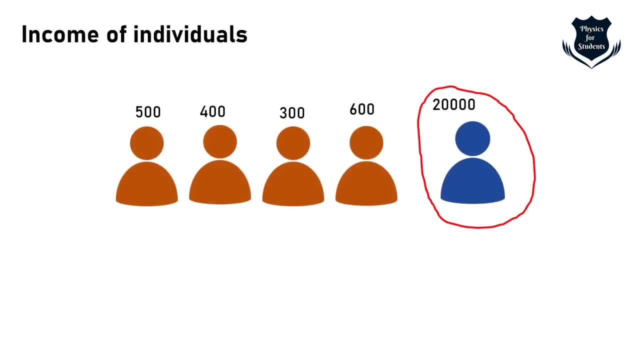 So here is the same individual: 500, 400, 300 and 600.. But here is something which I have marked in red in circle 20,000.. So we are going to calculate the average, But we are not going to take the arithmetic mean, or what do we mean by average? 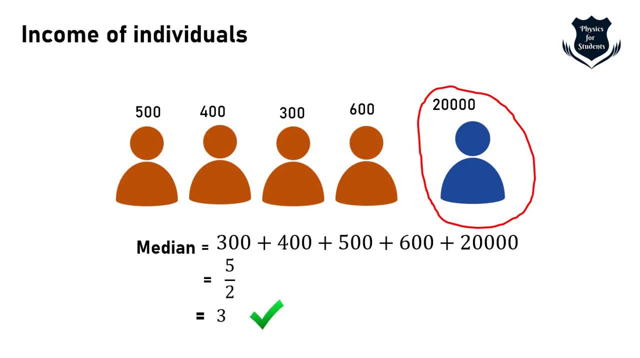 What we are going is that we are going to sum this up And we are going to divide it by 2. Which gives us 2.5. Which we can round up to 3.. So the position is here. So, in that case, if you really want to calculate the average of this particular series, 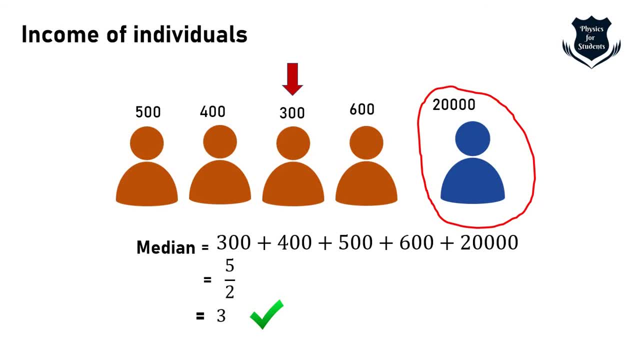 Where one individual which is marked in blue has got income Which is far more than what we can see right on here. We have to take the median, And here what we get is 3.. So we get the position 3, marked in red, as 300. 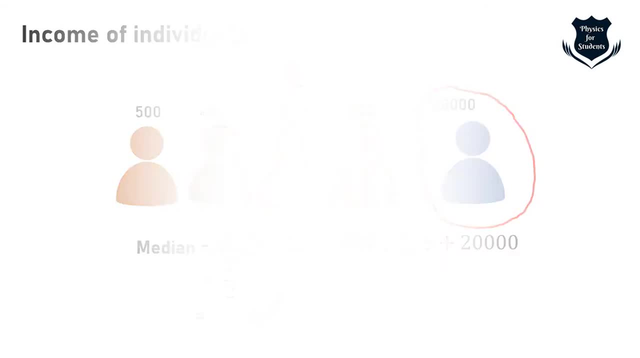 So this would be the median, So this would be the median. So in this kind of a case, we get a distribution: 3,, 5,, 7,, 6.. And another individual which is 9,000, which is more, And even if we get a smaller one, which is 50.. 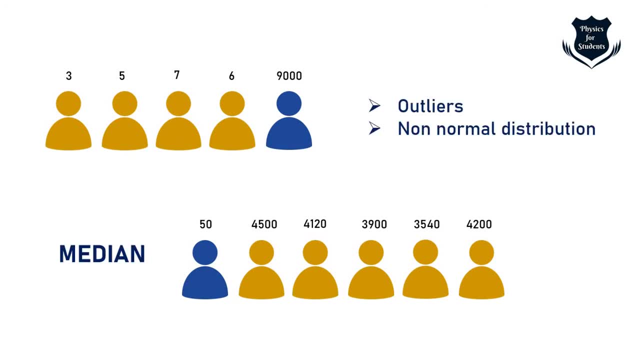 And we get this kind of a distribution. What we are going to do is that these 2 terms- This 9,000 and 50- are called outliers. That means they do not fit with the in general distribution of numbers that we have got. 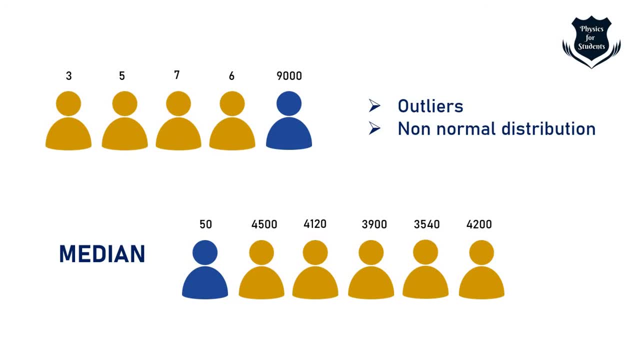 And it is also technically called a non-normal distribution. And if we get a economic distribution of this, a non-normal distribution, In this case we have to use median. So I have marked these two in blue so that you can understand which one is outlier and what is the method that we are going to use. 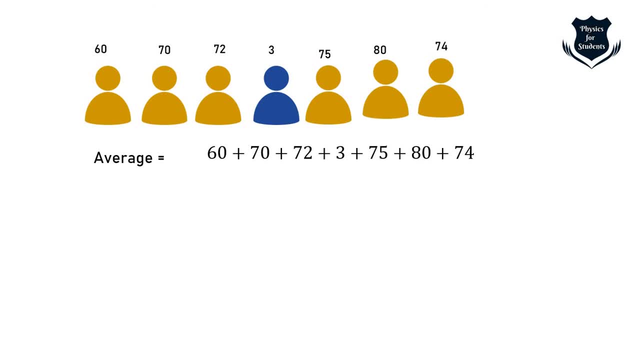 So let us take another example. So we get this series 60, 70,, 72,, 3,, 75,, 80 and 74. So this 3 one is the outlier which I have marked in red in blue, and when we take the average we get it is 62. 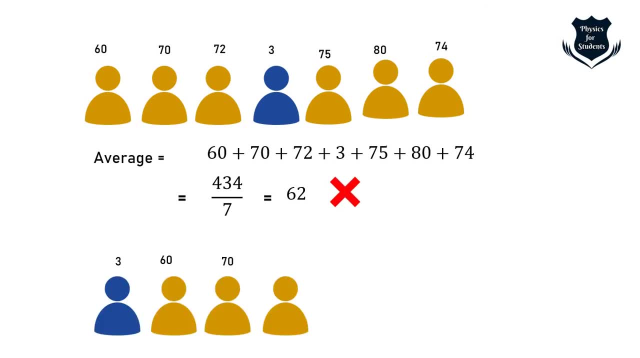 which is going to be wrong. Why? Because we have to do the same thing. First of all, we arranged it so in ascending order, So 360, 70, 72, 74, 75, 80, and then we take the number of occurrence. 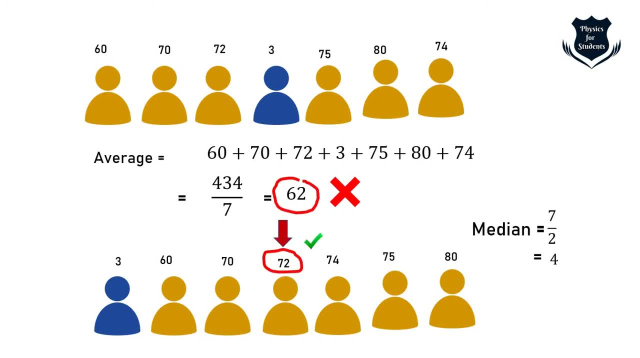 number, total number as 7, and we get 3.5, which is more or less 4.. Now you see that if it is 4, then the position and the value is 72, not 62. Now you might argue with me telling that, okay, fine, 62. and. 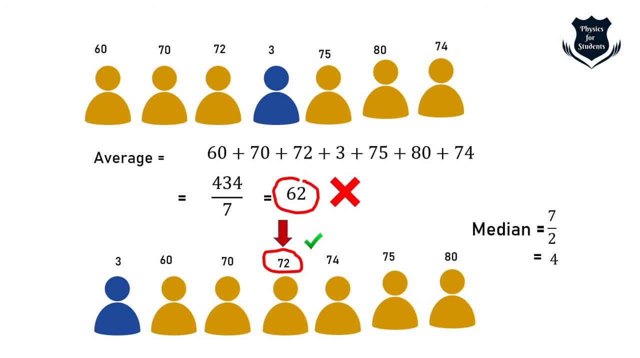 72 more or less is the same, but it is not. In case of long historical data or a long historical distribution of numbers or data. this is going to make the difference. So that is why the average calculation here the value- is 62, which is wrong. 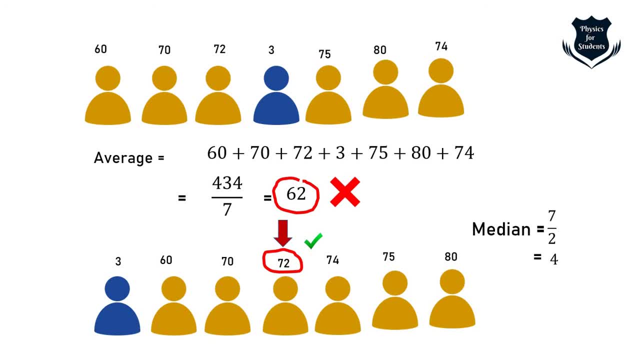 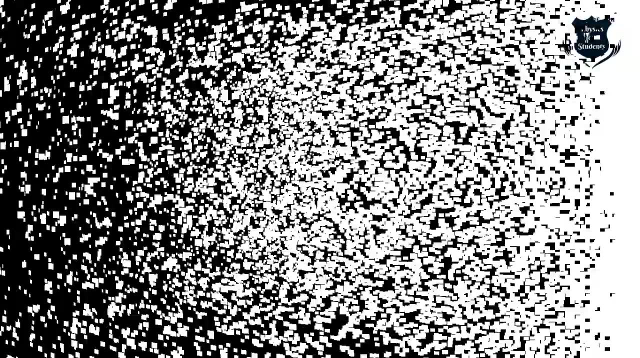 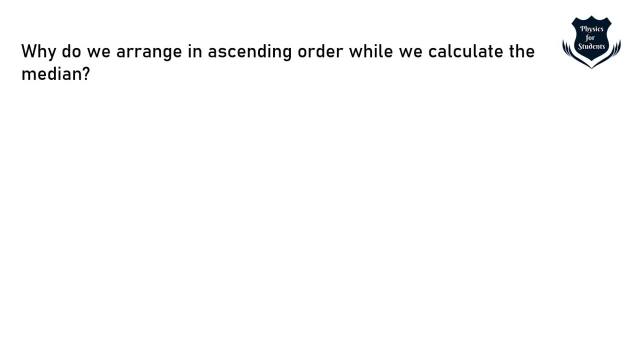 and here we have to use median, which calculates the value 72, which I have marked in green as tick marked. So here comes another important point, that why do we arrange in ascending order? while we calculate the mean, Well, we calculate the median. So here you see that here is a number, a series. I have given the blue, standing more or less in between, which is an outlier, and I have given the next series where, just on the just before, the final person, is another who is standing in as an outlier. So once we arrange them from ascending order, that is, from small, we go back to big. You see, I have marked this as red. 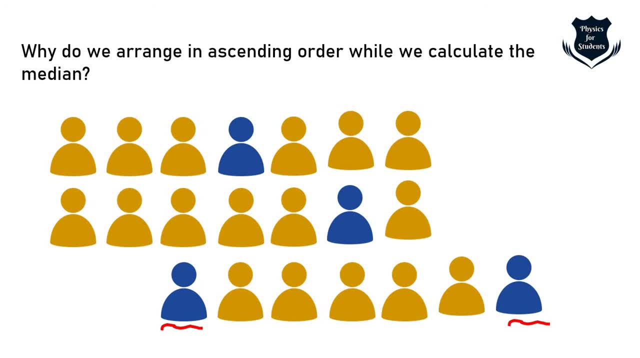 Why? because these two are outliers. and when we arrange, the beauty of using the median is that when we, when we arrange them in ascending order, these two which are marked on the left and the right as red arrow, these two, I would say, get extracted, these two values get out. 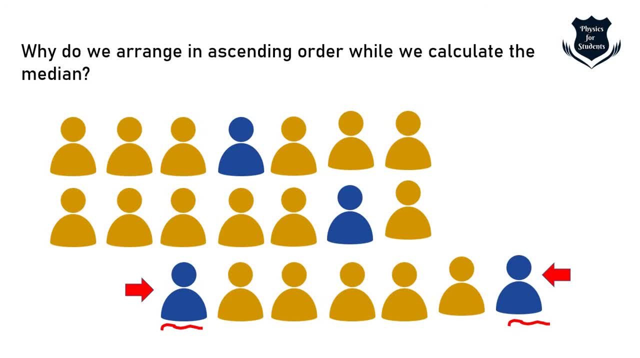 Right. So when these two start, two values are getting out. then there is no problem in terms of calculation of what we call median. So you see, once we calculate this, calculate the average, these two outliers would be included, which will give us a wrong answer when we are calculating using median. these two outliers are: 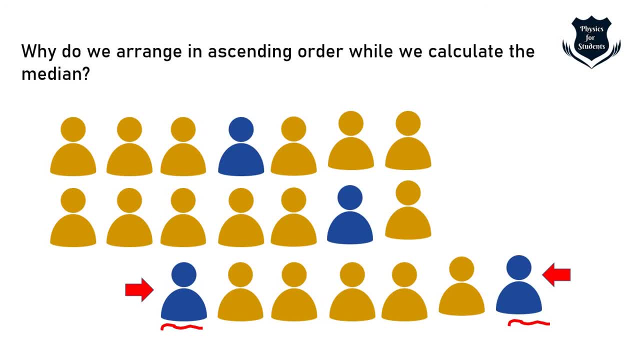 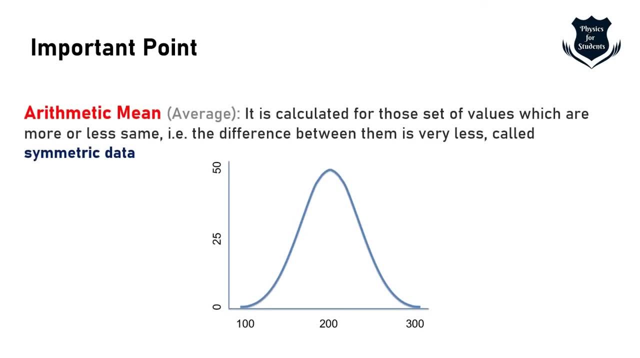 erased, they are taken out, so hence the calculation is not wrong. so one important point: we have to remember that while calculating arithmetic mean, we use the term arithmetic mean in general as average. it is calculated for those set of values which are more or less the same. same means the difference between: 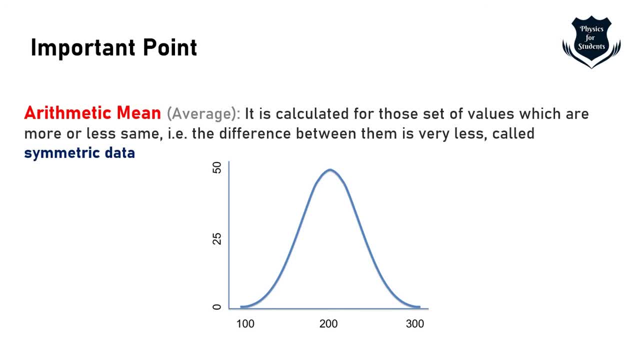 them is very less, as we have seen in the earlier example. technically it is called symmetric data, which is right there in front of your screen in blue. this is called a bell, bell-shaped curve which more or less can signify symmetric data. so we can use arithmetic mean which, again in a wrong notion, we call it as. 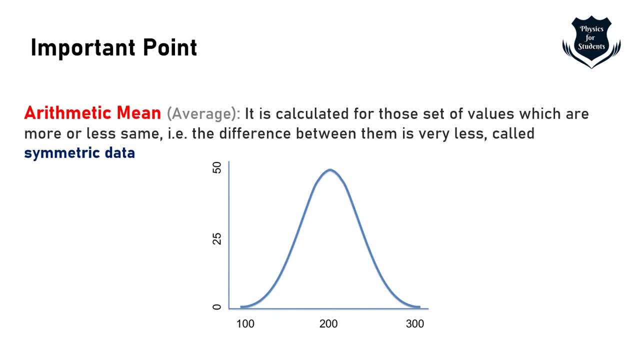 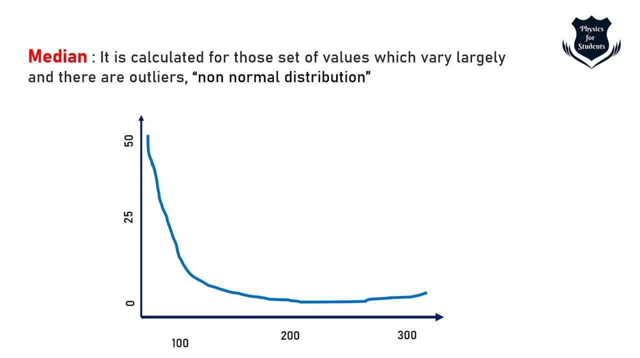 average on. on the other hand, when we are using median, it is calculated for those set of values which vary very largely. that means the differences are huge and they are called outliers, and here you see this blue one. this is a non-normal distribution. and in case of a non-normal distribution, or when we are getting a value where the 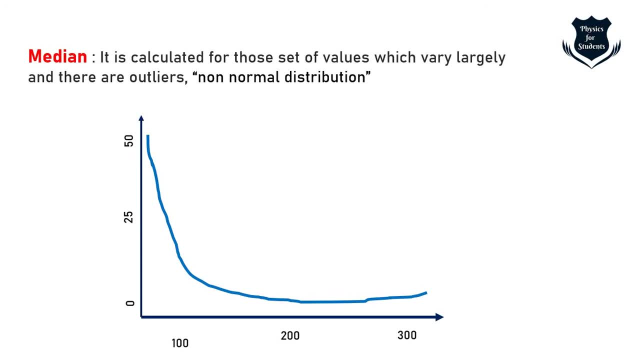 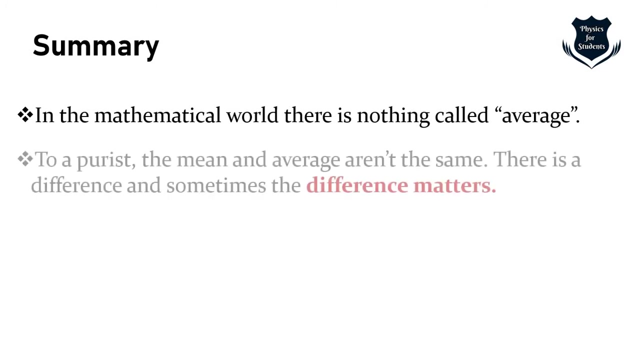 set or the series where the values are marks quite a big difference. we should not use arithmetic mean. we should use median to get the right value. so we come to the end of the video. just a quick summary on what we learned in the mathematical world. there is nothing called average. it is very misleading to 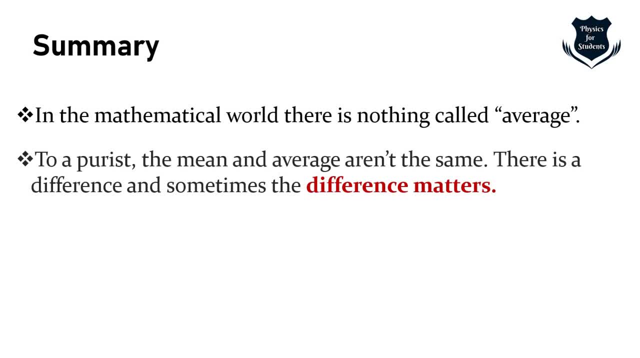 a purest, the mean and average. although they are the same, there is a difference and sometimes the difference matters. for normal distribution, that means for a, symmetric data where the value is not ranging or there is not much of a difference. we use a for non-normal distribution, asymmetric data, where the values are changing quite 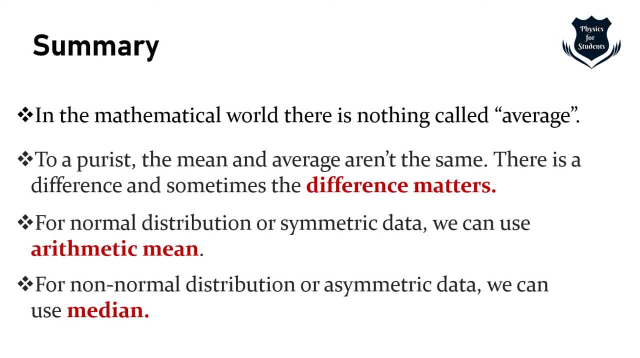 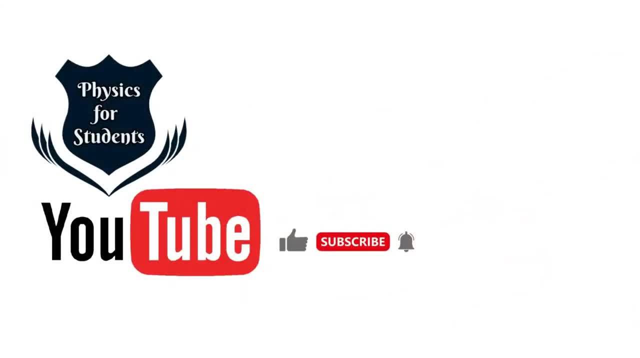 a lot. we can use median. thank you very much for watching this video. so just to summarize, as you can see, physics for students every time, every Sunday, is bringing up something new for you, so this video gives us a clear understanding. so the difference between average and mean. so what is that? by average we actually mean arithmetic.